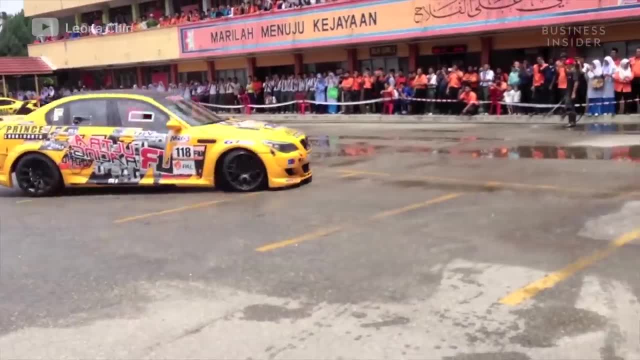 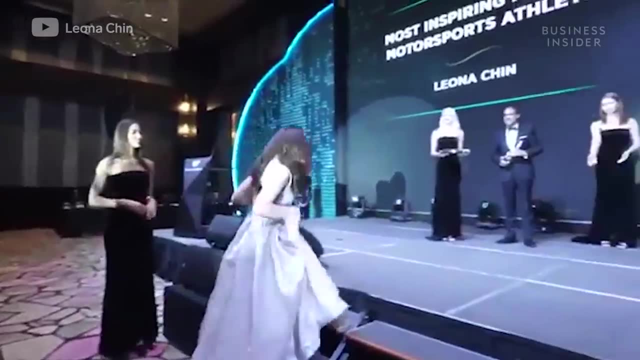 in rally, circuit racing, endurance racing, gymkhana, autocross, drag, off-road and go-kart. She's the driver behind mega-viral prank videos and the most inspiring female motorsports athlete, as voted by the Motorsports Association of Malaysia. 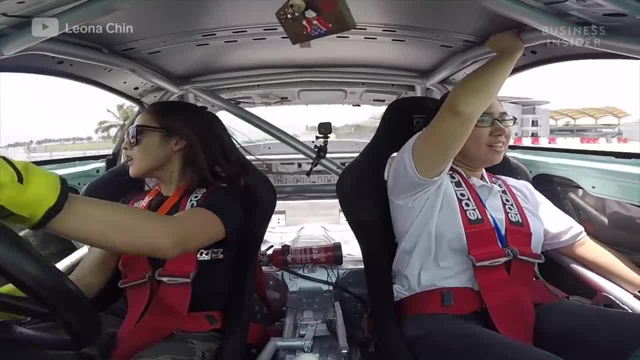 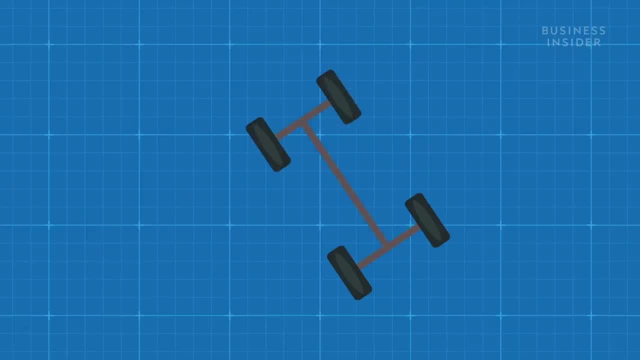 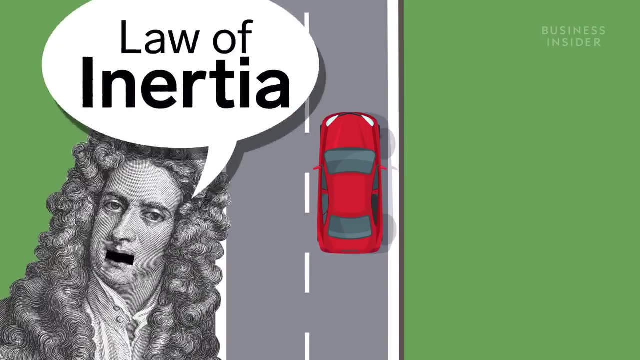 To those who know of her motoring exploits. she goes by another name: The Queen of Drift. Leona helped us understand how drifting works from a science perspective. According to Newton's first law, it's the law of inertia that states that when an object 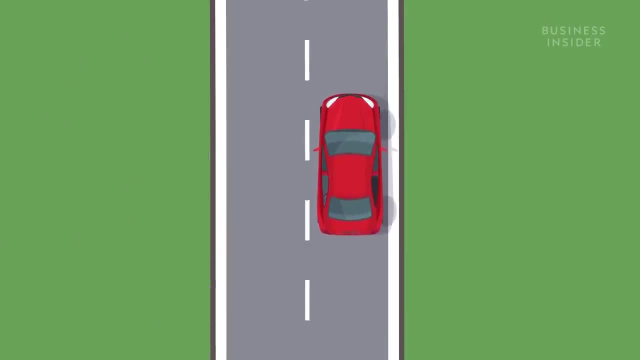 is moving, it wants to keep moving the same way and it resists any changes to that motion, unless there is an external force causing a change. Thus, in this case, the car's natural tendency is to go straight When the car's steering. 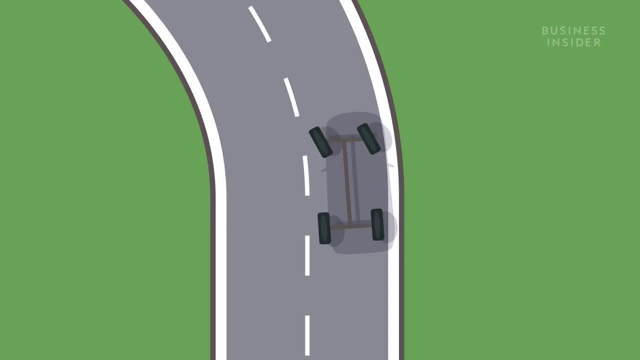 wheel is turned, then there is an external force. That force is the friction between the tires and the track, also called traction. When you turn the wheels, some of that traction is angled perpendicular to the car's velocity. So instead of moving in a straight line, the car begins to follow a curved path. 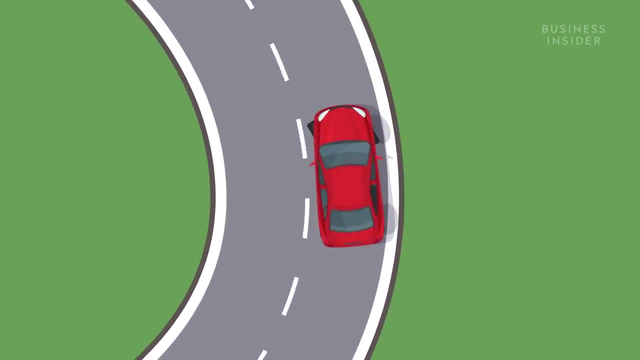 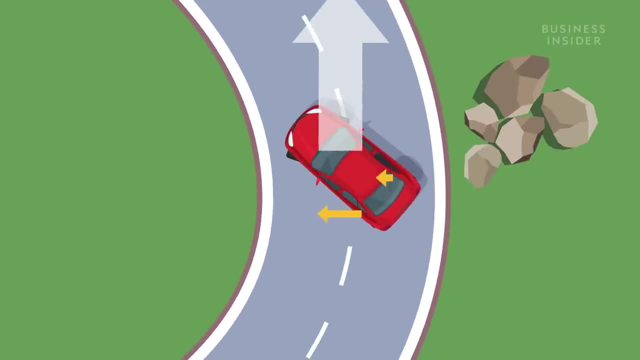 But this is not drifting. This is what happens during a normal turn. So when does a turn turn into a drift? When you overcome the friction between your tires and the road And you do that by entering a curve at an unusually sharp angle or an 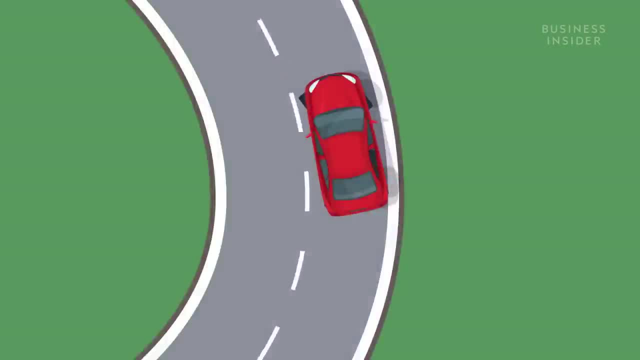 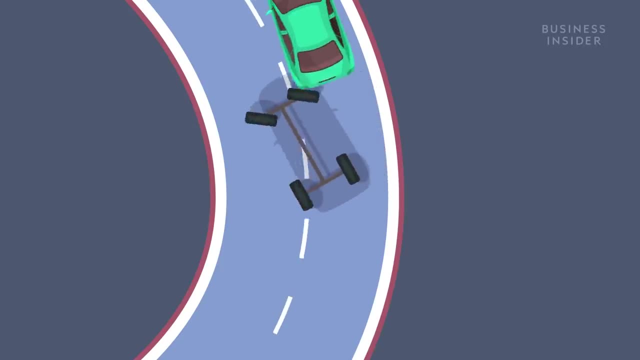 abnormally high speed. Think of a car moving on a surface where the force of friction is very low, Like on ice. A driver may turn their tires in order to avoid an obstacle like a stopped car, But the traction between the ice and the tires, 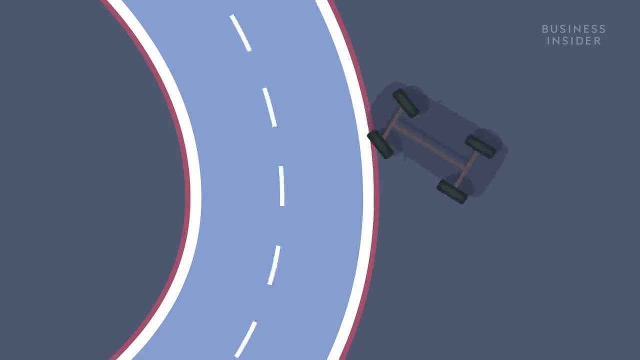 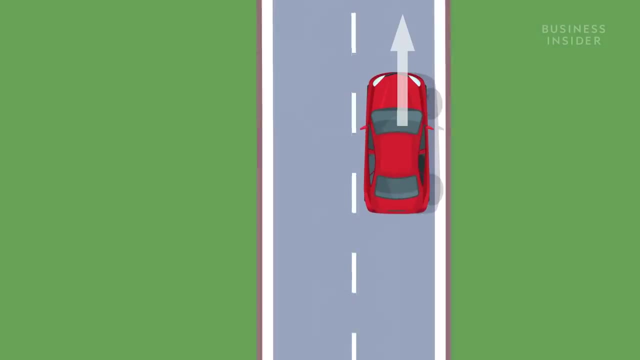 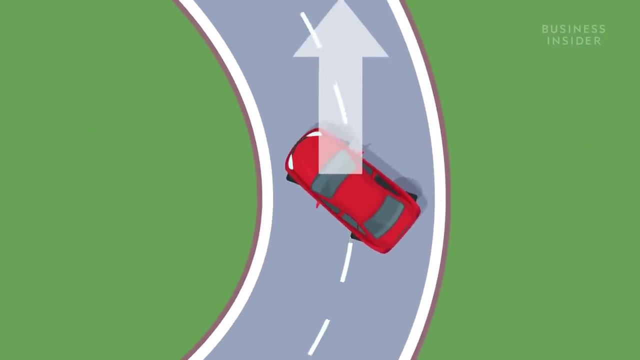 is so low that it's easy to overcome it. The car is in a slide. The same thing happens when a driver takes a curve too sharp or too fast on an asphalt racetrack. Now, a regular driver probably wouldn't know what to do during a slide and would likely.